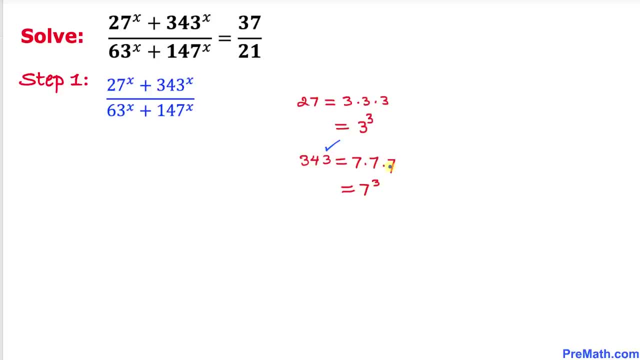 could be written as equal to 7 times 7 times 7, which is equal to 7 power 3. and now let's focus on in the denominator 63, and here I have copied down 63, this could be written as 9 times 7, which is equal to 3 times 3 times 7, which is equal. 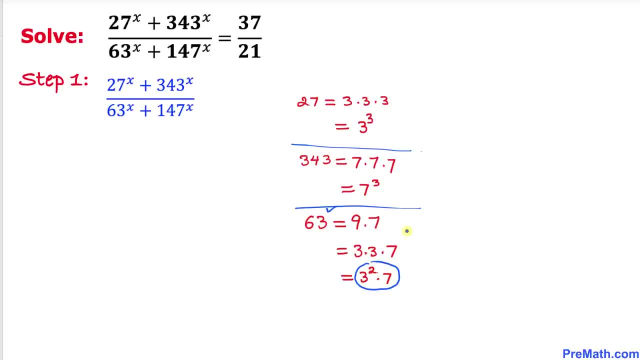 to 3 power 2 times 7. and finally, let's focus on 147, and here I have copied down 147, and if we put in a prime factorization, this could be written as 3 times 7 power 2.. So now let's revert back our attention to our this original. 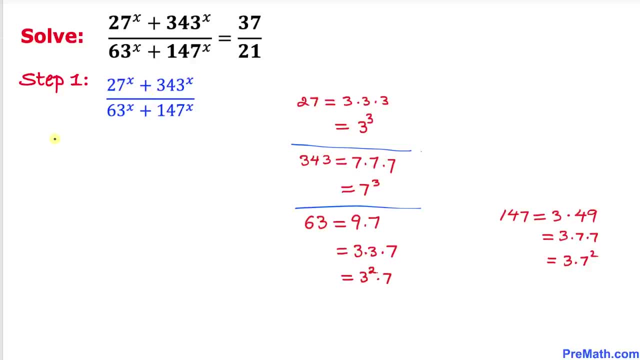 problems to 27. power X could be written as: 3 power 3 times 7 times 7, which is equal to 7 times 7.. 3 and then power X, and then plus 7 power 3 and then power X and divided by in the. 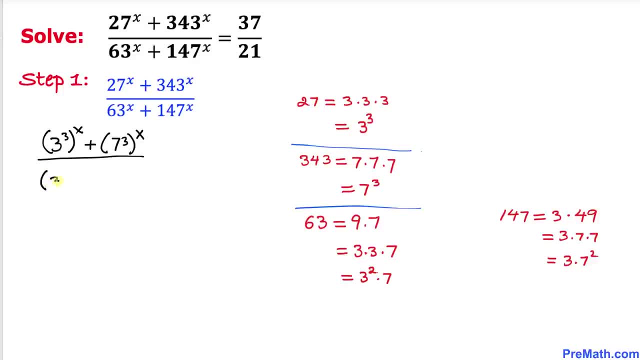 denominator 63 could be written as 3 power 2 times 7, and then power X plus 147 could be written as 3 times 7 square, and then power 3 times 7 and then power X in the denominator power x. now, before we go any further, let's focus on this. rules of exponent. we have got these nested. 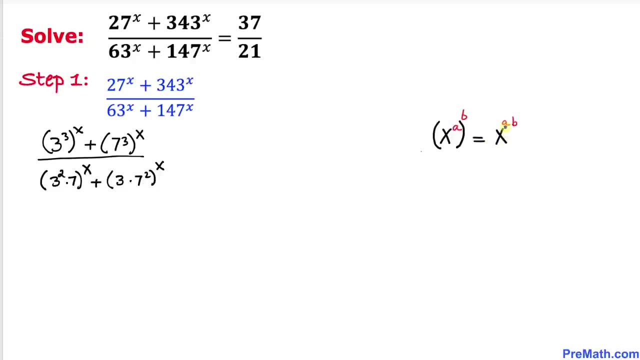 exponent x, power a and then power b could be written as x power a times b, and if we switch the exponent, if i write x, power b and then power a, this is equal to x power b times a. and just keep in your mind that a times b and b times a are same thing. therefore, these right hand side are: 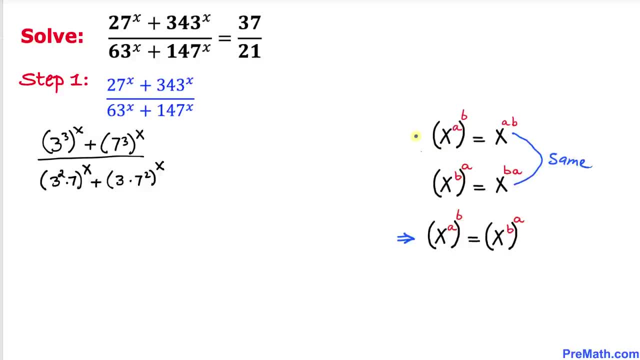 same. therefore, we conclude that these left hand sides are going to be same as well. now we are going to apply this rule on these numerator parts, so this could be written as 3 power x and then whole you, you, power 3, likewise plus 7 power x and then power 3.. Now let's focus on the denominator Over here. 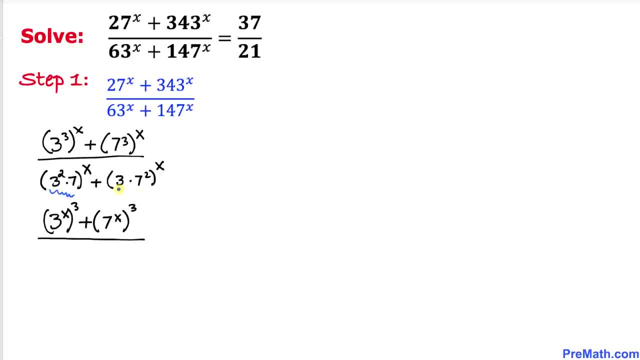 we can see 3 power 2 times 7 and 3 times 7 power 2. We can see that 3 times 7 is in common. So therefore we can factor out 3 times 7 whole power x, and then we are left with 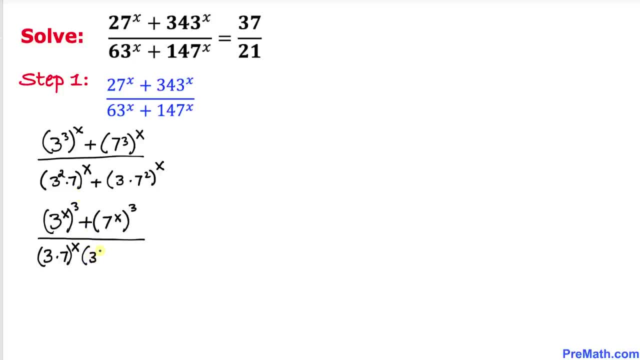 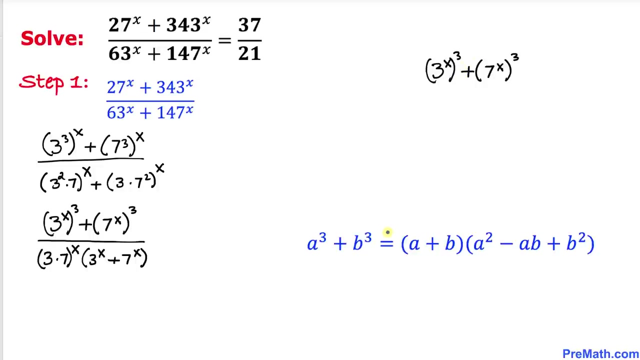 in the parentheses as 3 power x plus 7 power x. And now let's focus on the numerator part, only this one, And here I have copied it down and let's go ahead and take care of it, and we can see that we have a sum of two cubes. Therefore, we are going to use this well-known identity. 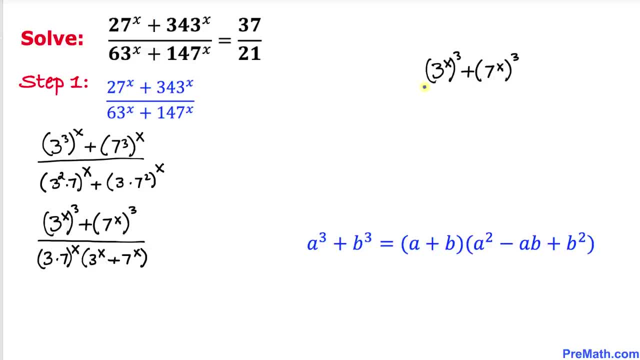 a power 3 plus b power 3.. So this whole thing could be written as 3 power x plus 7 power x and then times. we can write this one as 3 power x and then whole square. minus 3 power x, times 7 power x and then plus 7 power x, whole square. So let's go ahead and 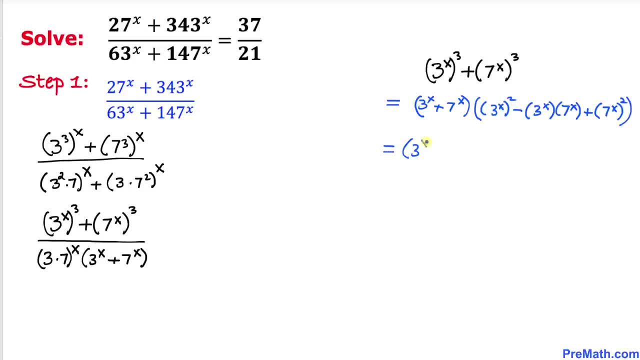 simplify it. furthermore, I can write this one just simply: 3 power x plus 7 power x, and here we're going to be using our rules of exponent. So this is same as 3 power. We have a nested exponent. We are going to multiply them, So 3 power, 2x and then minus. I'm going to leave that one. 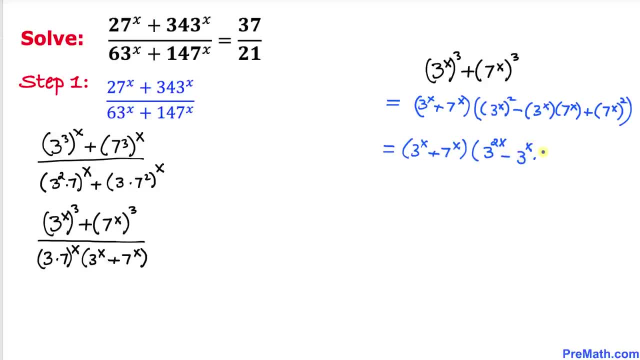 as it is 3 power x and then times 7 power x and then plus 7 power 2x. So our this numerator is going to be simply: we are going to replace this one, So I can write this one as 3 power. 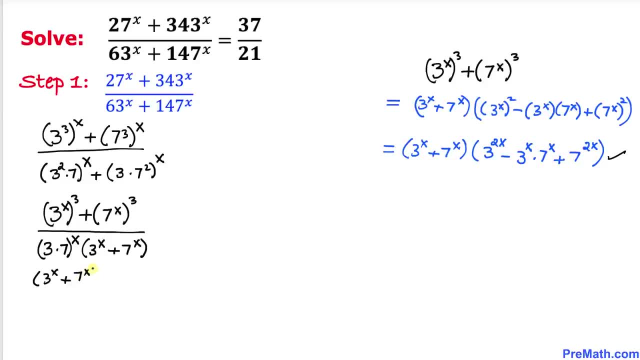 x plus 7 power x times 3 power 2x minus 3 power x times 7 power x. and then plus 7 power 2x. on the numerator, Now let's focus on the denominator. This 3 times 7 power x could be written as by: 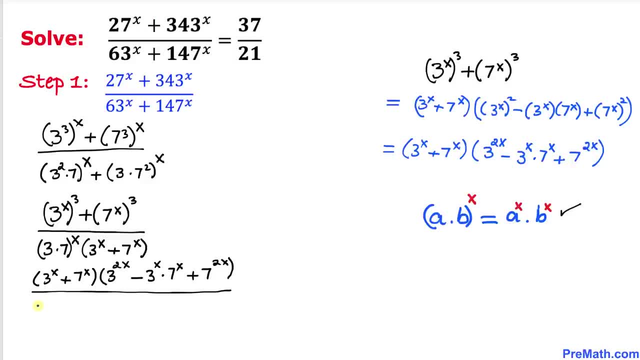 using this rule. So this could be written as 3 power x times 7 power x, and then in parentheses, 3 power x plus 7 power x. Now we can see that these factors, 3 power x plus 7 power x, and this denominator- they cancel each other out. 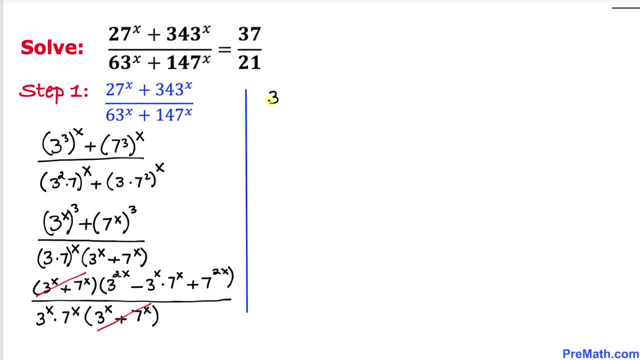 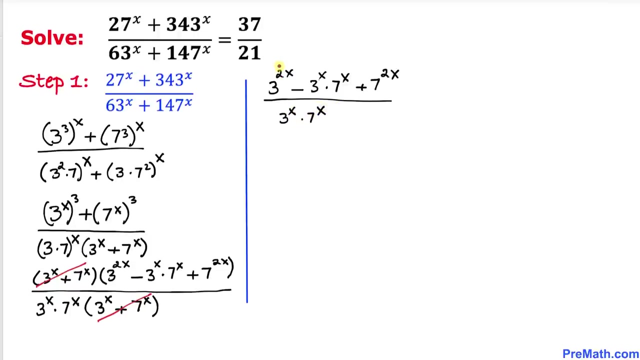 Therefore, our simplified fraction is going to be 3 power 2x minus 3 power x times 7 power x plus 7 power 2 x, divided by 3 power x times 7 power x. and now let's focus on this part: 3 power 2x. and here I have copied down 3 power. 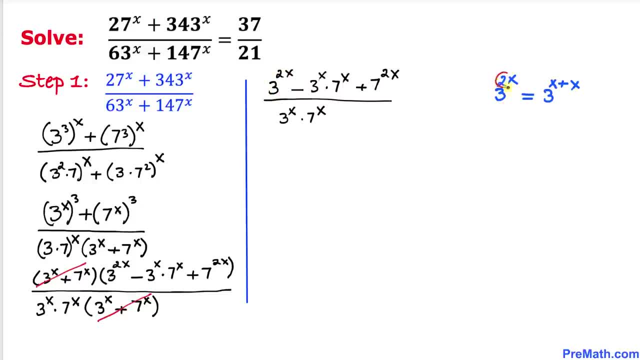 2x right up here, and its exponent, 2x, could be written as x plus x, and now we are going to use this product rule, so therefore, this could be written as 3 power x times 3 power x, and likewise- let's focus on this- 7 power 2x and I. 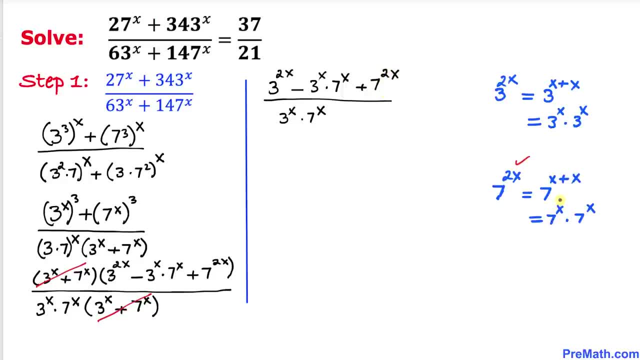 have copied it down over here, and this could also be written as a 7 power x times 7 power x. therefore, our numerator could be written as 3 power x times 3 power x. minus 3 power x times 7 power x and plus 7 power x times 7 power x divided by our 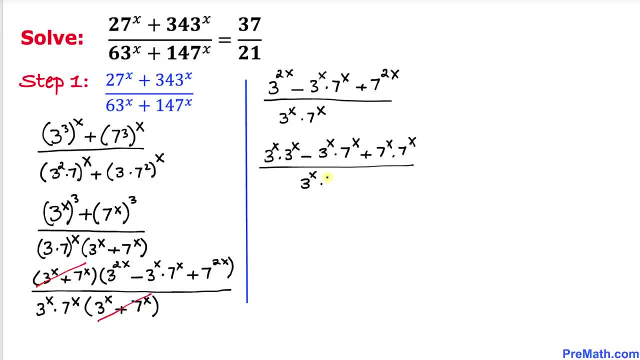 denominator is 3 power x times 7 power x. in this next step, I have divided this common denominator by each and every term. by using this rule, now we can see that 3 power x and this 3 power x cancels out, and here 3 power x, 3 power x is got. this fraction could be: 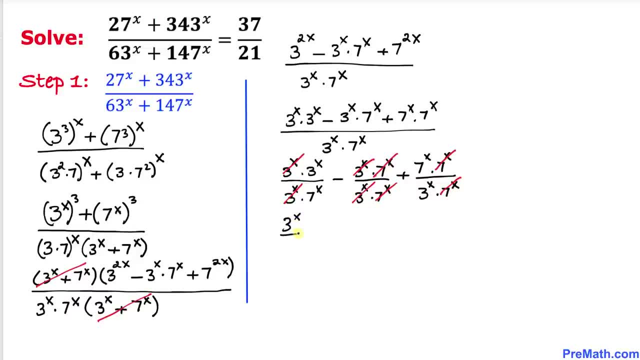 simplified as 3 power x divided by 7 power x, and here we got just simply negative 1 and plus 7 power x divided by 3 power x. therefore, we can write this one, 3 divided by 7, whole power x, by using this: 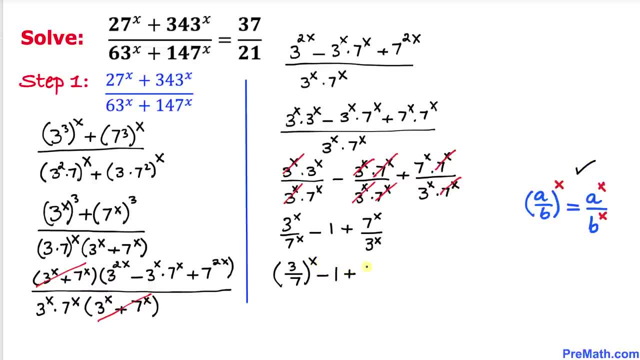 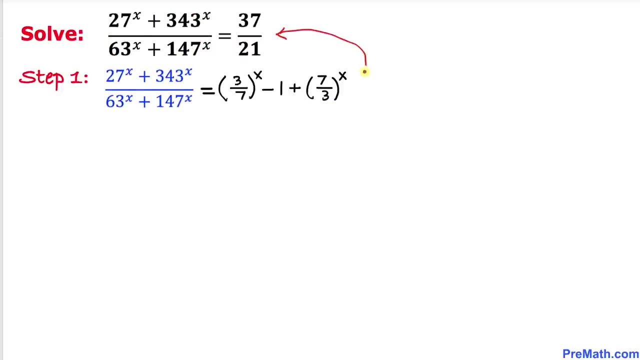 rule, and then minus 1 plus 7, divided by 3, power x, and now we can see that our this left hand side has been simplified to this form, so I am going to replace this left hand side by this. so, therefore, we are going to equate these right hand. 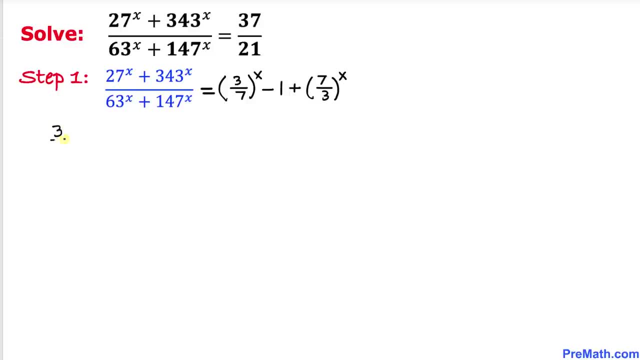 sides. that means this: 3 divided by 7, whole power x minus 1 plus 7 divided by 3, whole power x equal to 37 divided by 21. and now let me go ahead and call this as an equation number 1, and here's our 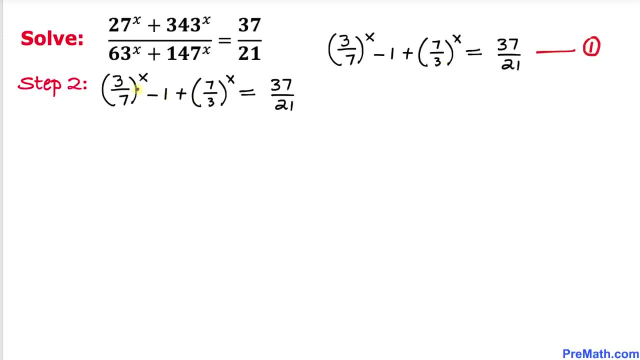 next step, let's focus on this equation 1, that I have just copied it down and we want to make things simple, so let me go ahead and make a substitution. I am going to call this part as a. you know, you go ahead and write down: let you equal to 3 divided by 7. 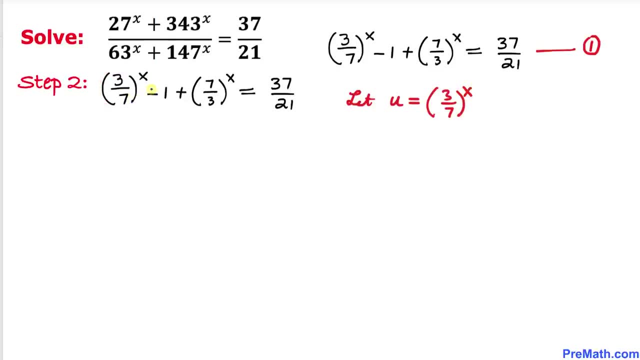 power x. Therefore, i would this: given equation is going to become a: simply you minus one plus. let's focus on this part, and here this seven divided by 3 power x could be written as 1 over 3 divided by 7 power x, and we know that this is u, so this: 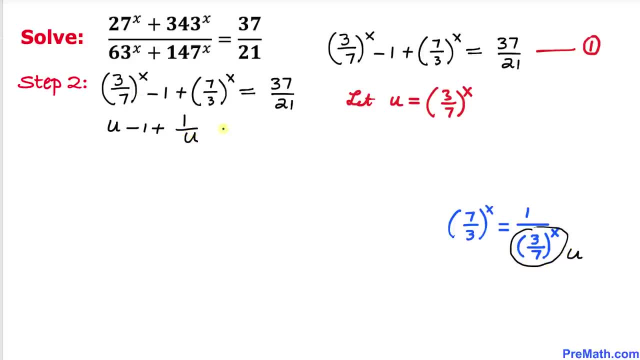 could be written as: plus 1 divided by u equals to 37 divided by 21.. Now let's go ahead and remove the fraction. so I'm going to multiply both side by u, on the left hand side and on the right hand side as well. So let's go ahead and distribute these ones, so that's going to be u square minus. 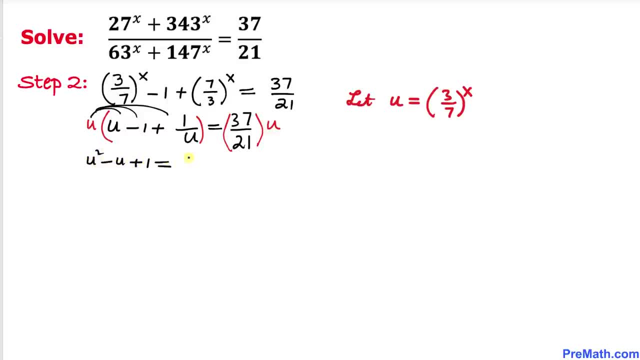 u and then plus 1, equal to 37 u divided by 21.. Now let's get rid of this 21 from the denominator. so I'm going to multiply both side by 21 on this side and 21 on this side as well. So let's go ahead and. 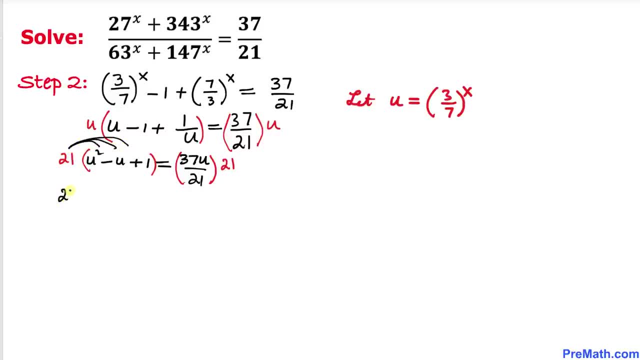 distribute once again, So that is going to give us 21 u square minus 21 u plus 21 equals to this 21. 21 is gone, so we ended out with 37 u. Now let's go ahead and subtract 37 u from both side, so this could be written as: 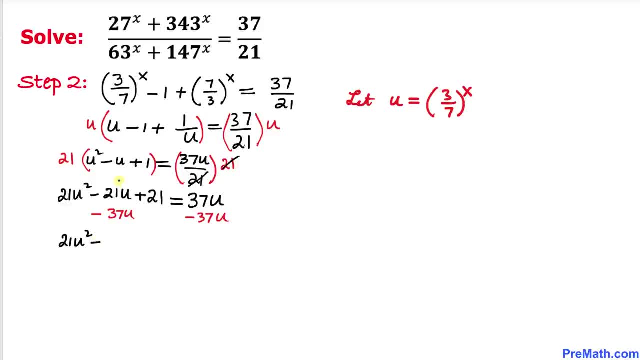 21 u square, and that is going to give us negative 58 u. So let's go ahead and subtract 37? u plus 21 equals to. they cross each other out, so we have equal to zero. and now we can see that this is our quadratic equation and we are going to solve by factoring. We could also 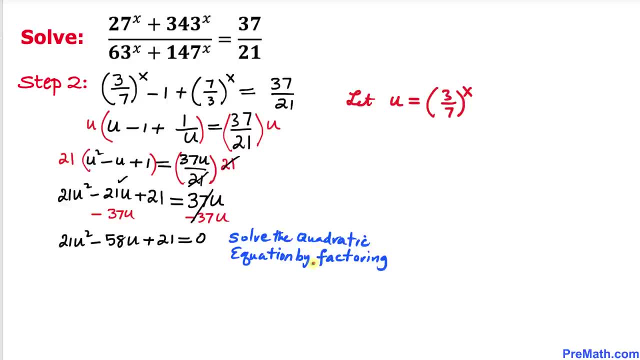 solve by using quadratic formula, but I think factoring is going to be a lot more easier, So let's tweak this part. negative 58 u could be written as negative 9 u minus 49 u. Let's go ahead and write down 21 u square minus 9 u minus 49 u. plus 21 equals to 0, and now we can see: 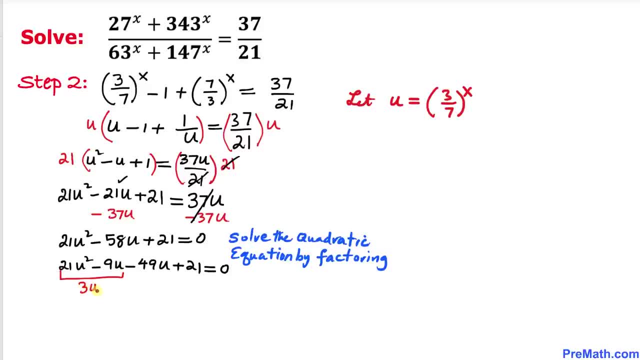 there's a 3? u is in common between these two terms, and over here seven is common from these couple of terms. let's go ahead and factor out 3? u from here. we got 7? u minus 3, and here let's factor out 7. so we got in parentheses 7? u minus 3, equal to 0, and now we can see that 7? u minus 3. 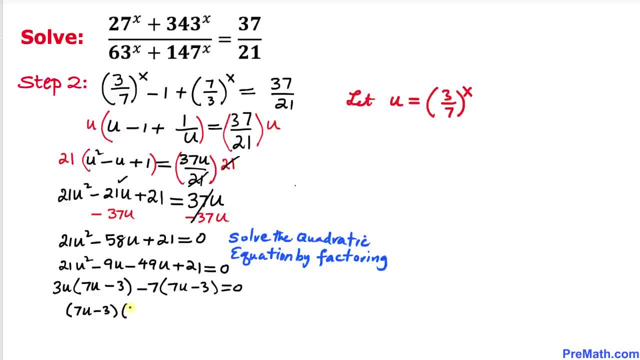 is in common. I can put it in a factor, and then 3 u minus 7 equals to 0. now let's go ahead and separate these factors, so I can write 7 u minus 3 equal to 0, and on this side, 3 u minus 7 equal to. 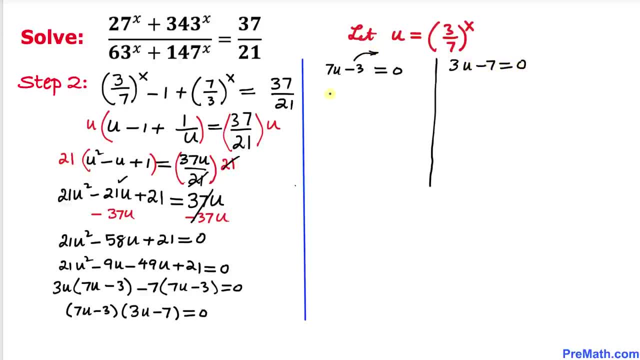 0. now let's go ahead and move this negative 3 on the other side, so 7 u equal to positive 3. so u turns out to be 3 divided by 7. and likewise we're going to be moving this negative 7 on the other side, so that means u turns out to be 7 divided by 3. but we know that. 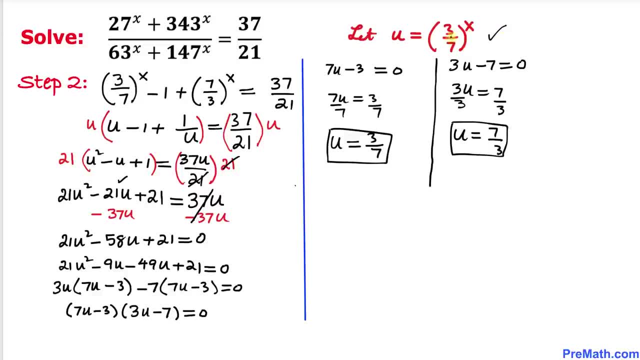 our u value that we substituted equals to 3 divided by 7, power x. let me go ahead and replace this one: 3, 3 divided by 7, whole power x for u. and on the right hand side we got 3 divided by 7. now 3 divided. 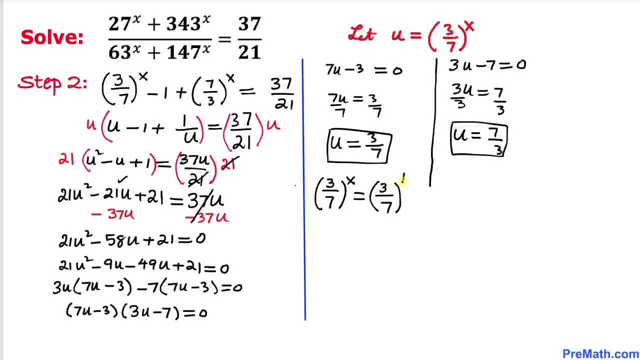 by 7 could be written as 3 divided by 7, whole power: 1. now we can see that our bases are same, so according to this rule, we can equate our these exponents. therefore, we can write: our exponent x equals to 1, and that is our 1 of the solutions. and now let's focus on the other value of u, which is 7 divided. 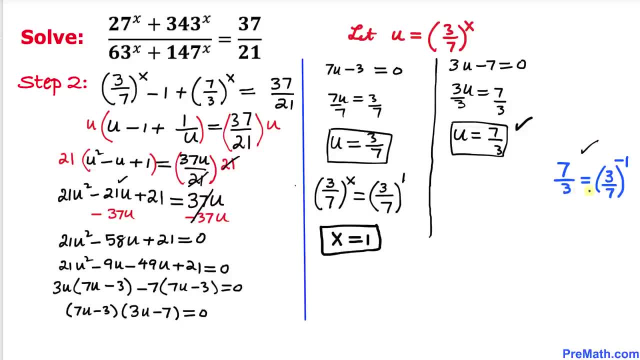 by 3, and we know that the 7 divided by 3 is same as 3 divided by 7, power negative 1. so therefore I can write this u as 3 divided by 7, whole power negative 1, but then our u value is 3 divided by 7. 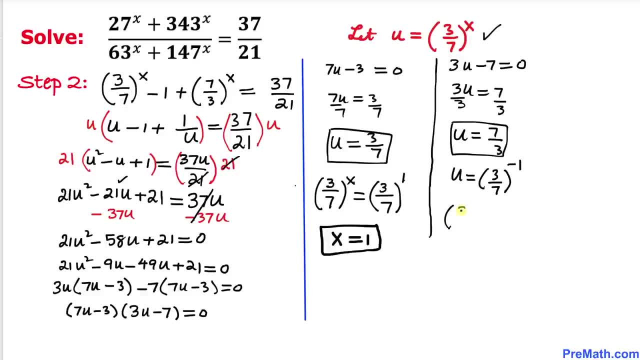 power x. let me go ahead and replace that one. so 3 divided by 7 whole power x equal to 3 divided by 7 whole power negative 1. and now we can see that our these bases are same. so therefore we can equate these exponents. so therefore we can write x equal to negative 1, and that is our another solution. so